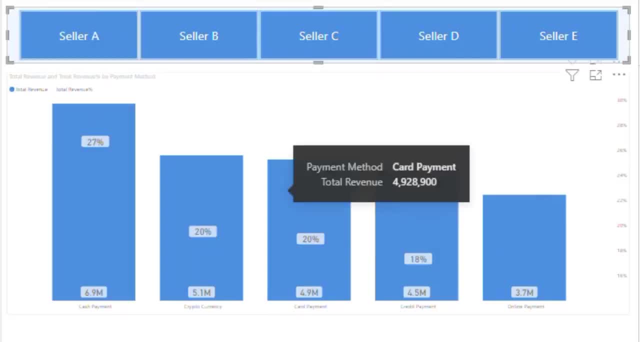 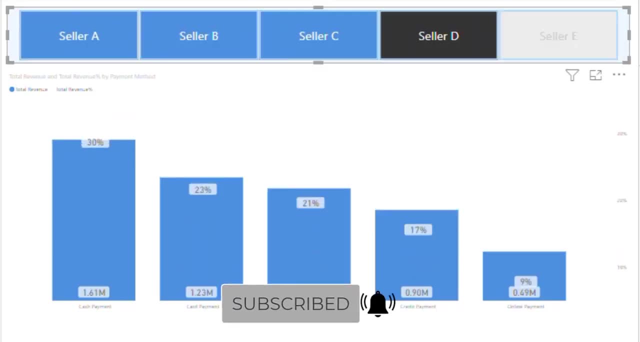 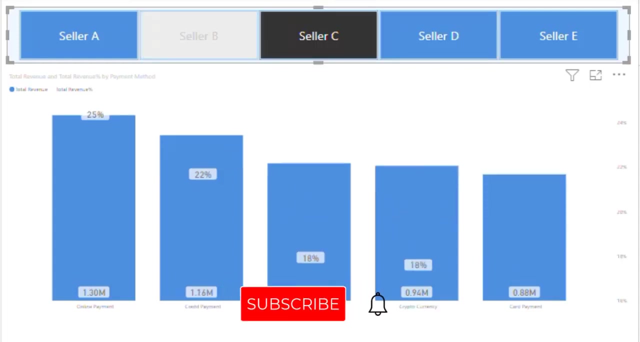 Hello and welcome to Sunday Power BI. Today, we are going to learn an awesome technique that allows you to create a bar chart displaying values as absolute number and as percentage of total at the same time. Remember, Power BI doesn't have a built-in visual that allows. 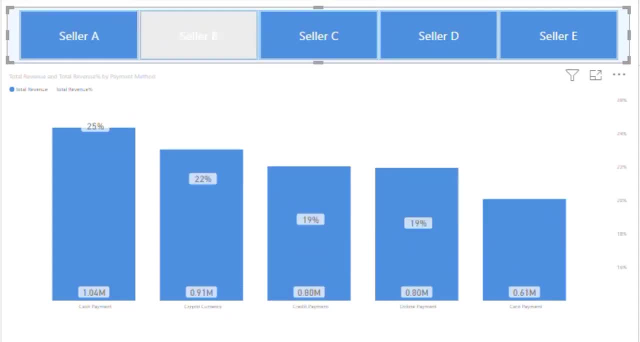 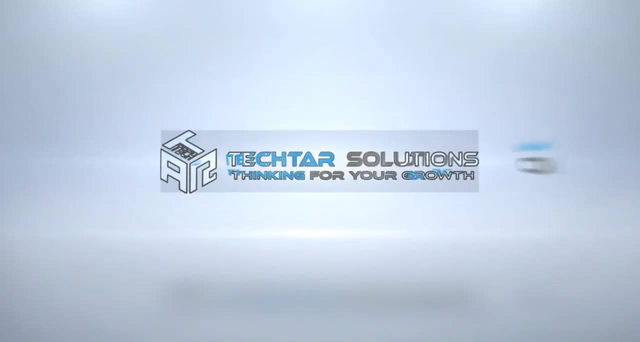 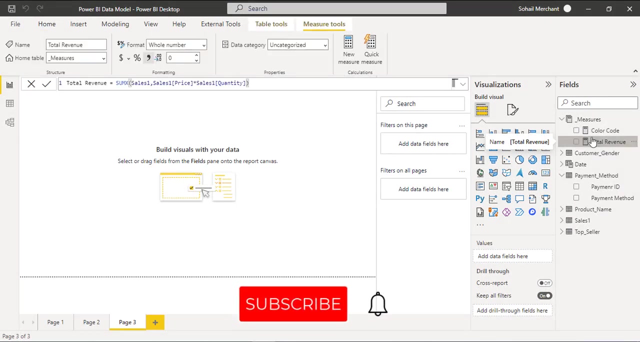 you to create something like that. So we are going to perform this technique in three simple steps. Let's start the video. I have already created the basic measure to calculate total revenue For percentage. we are going to create another measure using divide and calculate functions Right click. 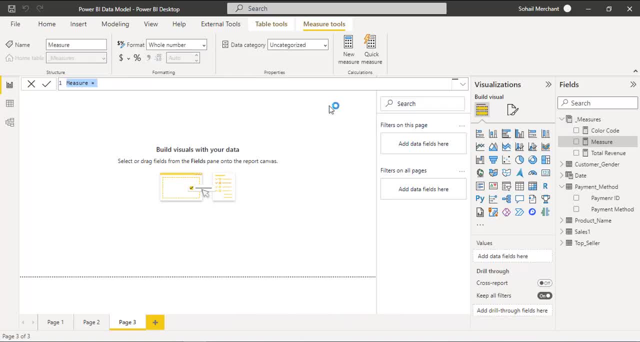 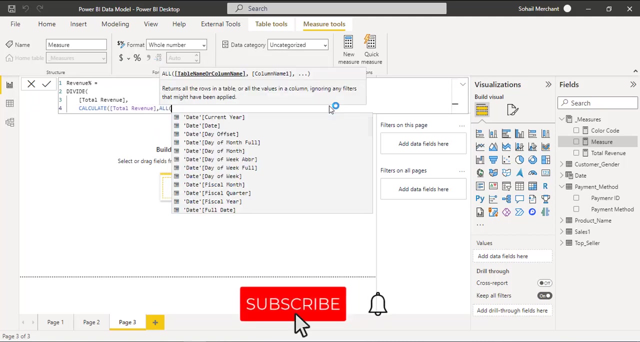 new measure and we are going to call this measure as revenue percentage divide. We want to divide total revenue By its grand total and for grand total we are going to use calculate function, Calculate total revenue all and since we are going to create this chart for payments, therefore, 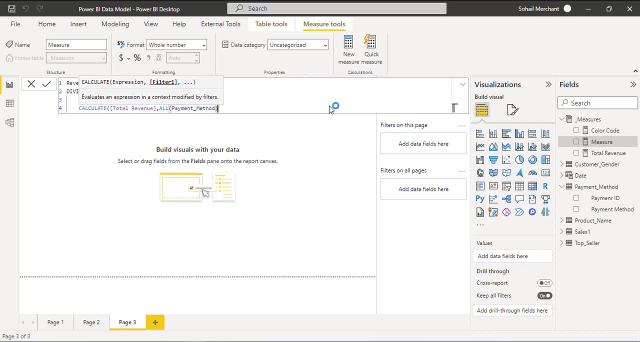 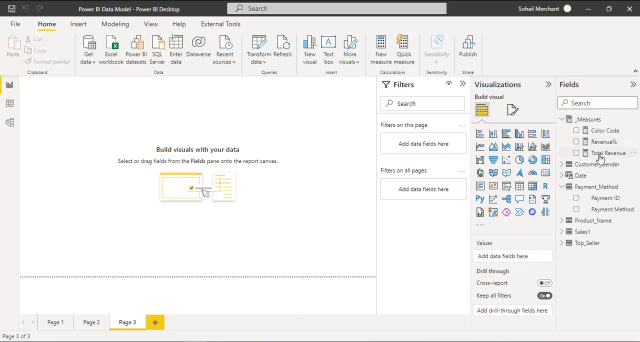 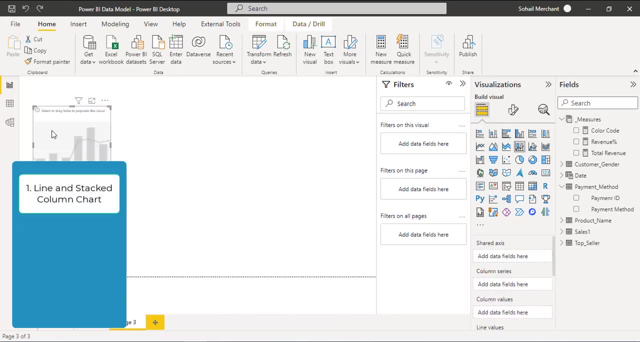 we are going to use payment method table. So we have both the measures in front of us, for percentage and for absolute values. Now the first step is to select line and state column chart. This chart gives you value for column and value for line. Resize it. Now we will drag the total revenue measure. 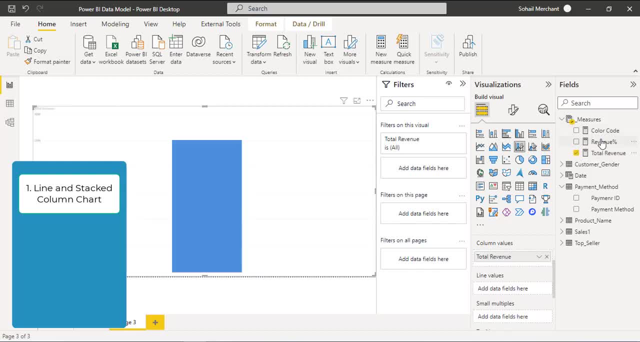 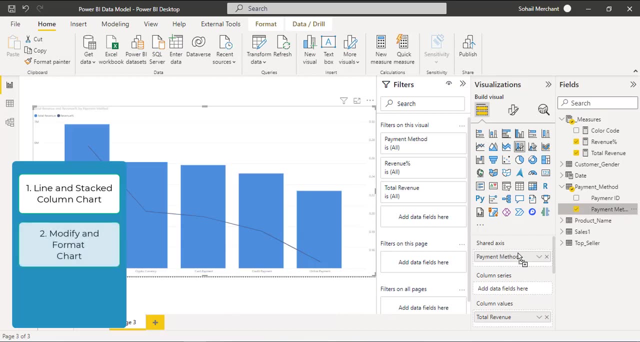 in column values and revenue percentage measure in line value. And since we want to show payment method on x-axis, therefore we are going to drag payment method on shared axis, So we are going to use payment method on x-axis. In step 2, we are going to modify this chart. 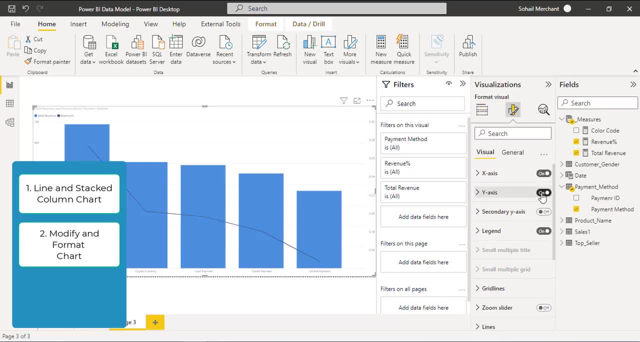 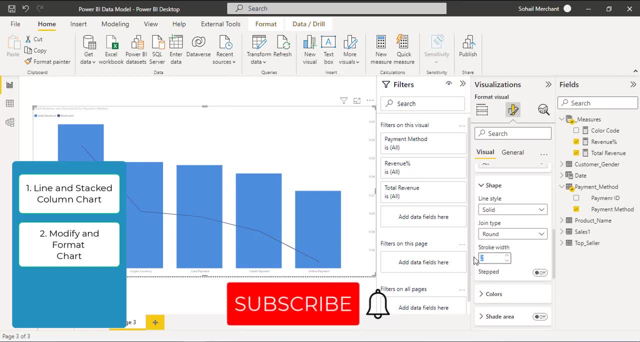 For that, click on format your visual option. Close y-axis From the lines option. mark your stroke width 0.. Line color matching your background color. that is white. That's it from the line. In last we are going to enable data label option From apply settings to. 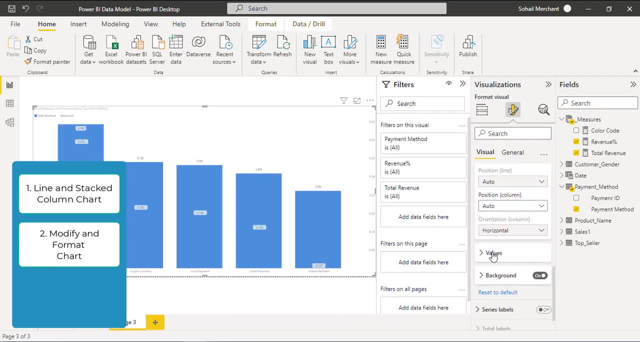 we will select our first measure: total revenue. We want to increase the value of our total revenue. We want to increase the value of our total revenue. We want to increase the font size of values. Click on values and change the font size from 9 to 15.. You can.